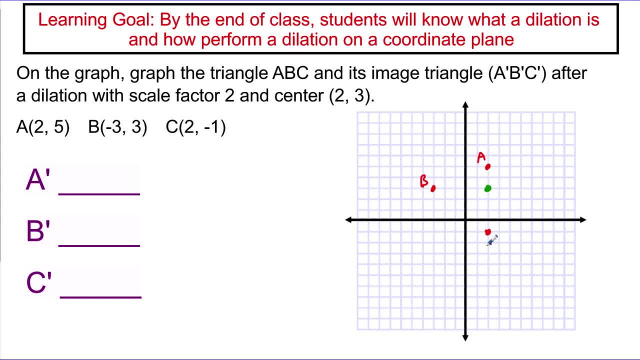 and I have the point 2 down to negative 1, and this is my C, and let's put those together using a red line. So I'm going to go A to B and B to C, And I'm going to go C back to A, and so let's figure out how this is going to dilate by a scale factor of 2.. 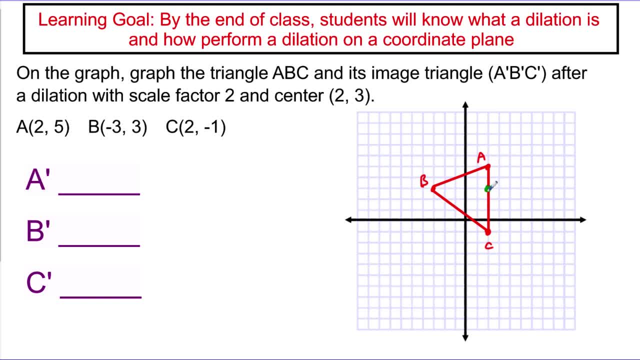 So if I'm taking a look, counting from my center of dilation, which is at 2,, 3, up to A, it looks like all I'm doing is I'm going up 1, 2 units But a scale factor of 2 means that I should double the distance that it was from that center. 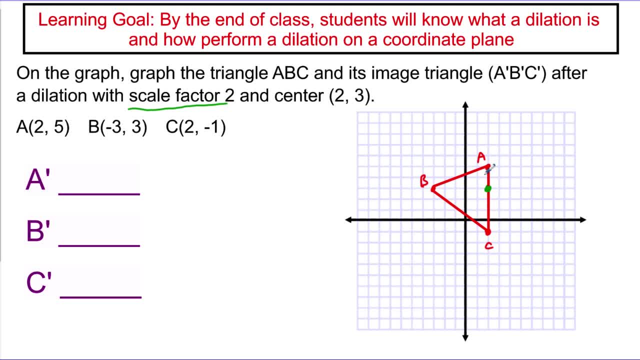 So I'm going to say, in this case, Instead of going up by 2, I should double how far I count. I'm going to go up by 2, and I'm going to go up by 2 again, and I'm going to end up right here. 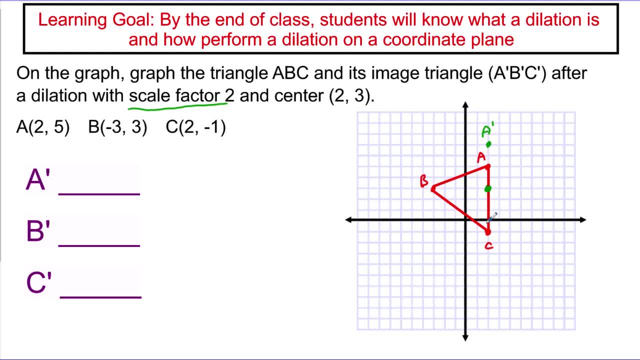 This is my new A prime, so let's just figure out what that point is. That's: 2, 1, 2, 3, 4, 5, 6, 7, the point 2, 7.. 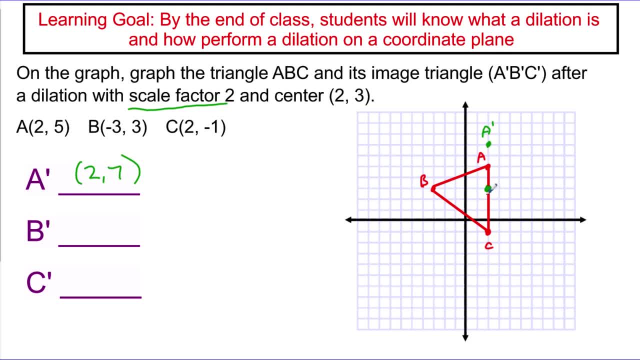 So that one's fairly straightforward because it's right on the same line. So I can do the same thing with C. If I go down 1,, 2,, 3,, 4, I end up at C. So what I'm going to do is I'm going to go down 4 again. 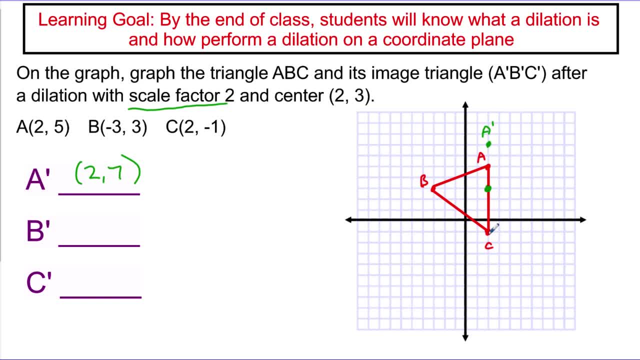 A scale factor of 2 means do that thing twice. So I'm going to go down another 4, 1,, 2,, 3,, 4, and I'm going to say my new C is down here And that looks like the point: 2, 1,, 2,, 3,, 4, 5, 5 down 2, negative 5.. 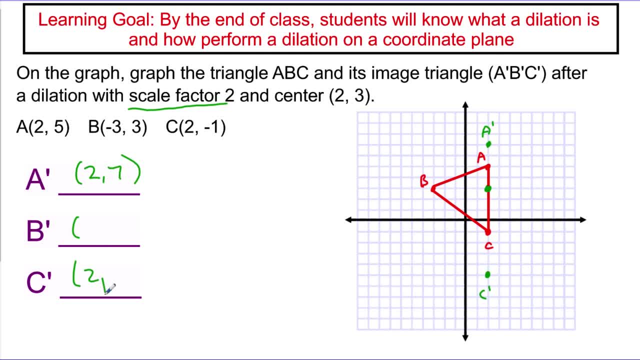 Oops, let's fix that. That's my C value: 2, negative 5.. And then I have one more B. B is a little bit more challenging, but it looks like to get to B, I go straight over 1, 2.. 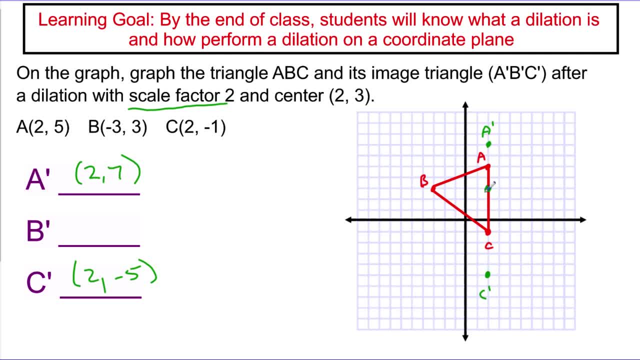 3,, 4, 5, OK, And so instead I need to do that twice. So I went 5 to get to B and I need to go another 5, 1,, 2,, 3,, 4, 5.. 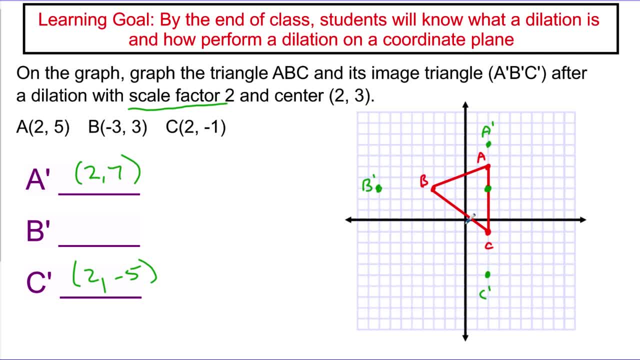 Now I'm twice as far away. This would be my B prime right. So I'm going to say, in this case this looks like negative 8, 2 instead. OK. So if you notice, there's no real algorithm here. 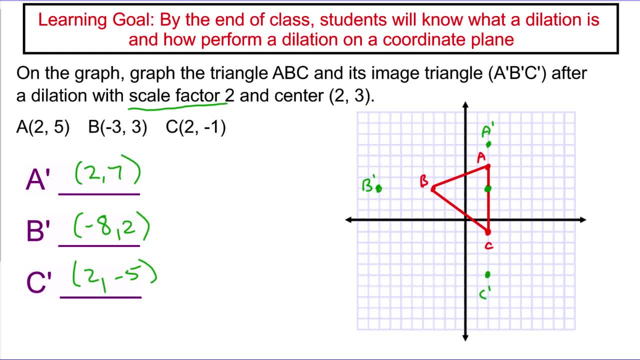 Because I'm changing my center of dilution to not be the origin. OK, I'm going to have to just count boxes and use what I know about scale factor right? So it looks like this: This would be my new ABC, OK, which again just kind of expanded my graph out and it pushed some of my values away from that center of dilution to its new point. OK, 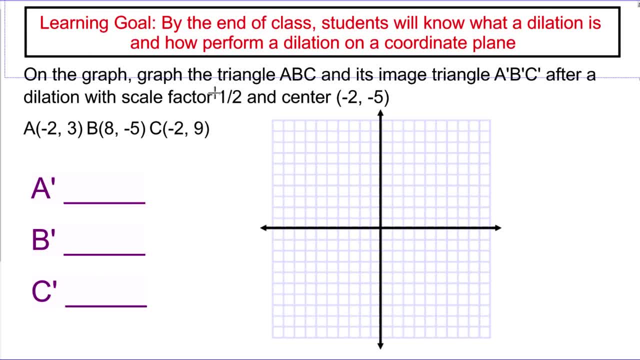 So let's take a look at another one which maybe, in this case we're doing a dilution of 1 half instead of 2.. So I'm going to first plot my center of dilutions, which is at negative 2, and then down 1,, 2,, 3,, 4,, 5.. 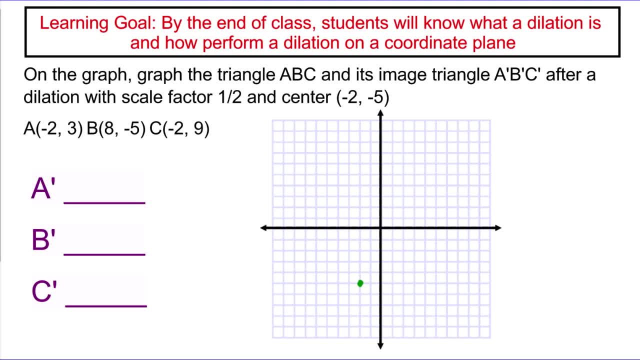 That's right here. OK, So this is my center of dilution And I'm going to plot each of my points, which is negative, Negative, 2, up to 3, right. Same negative: 2, 3, right. 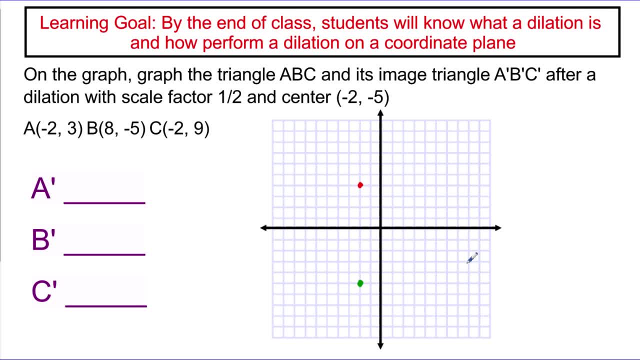 And then I have 8, up to or down to 5.. 1,, 2,, 3,, 4,, 5, OK, And then negative 2, all the way up to 9, OK. So let me do those in order. 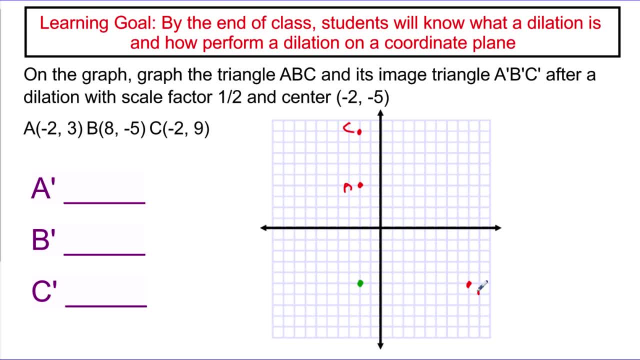 So this is A and C, and B is way over here, So let's connect those together. We want a nice triangle, OK, So this is going to be my triangle ABC, OK, and our job is to scale this down by a factor of 1 half using the center of dilution over here. 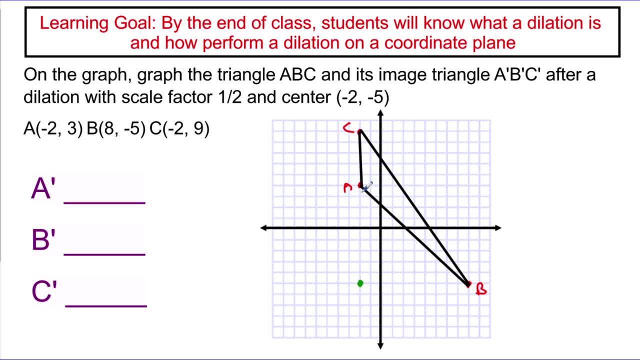 OK. so what I'm looking at now is, when I count up to A, I'm counting 1,, 2,, 3,, 4,, 5,, 6,, 7,, 8.. Let's try that again: 1,, 2,, 3,, 4,, 5,, 6,, 7,, 8,, 9 units up. 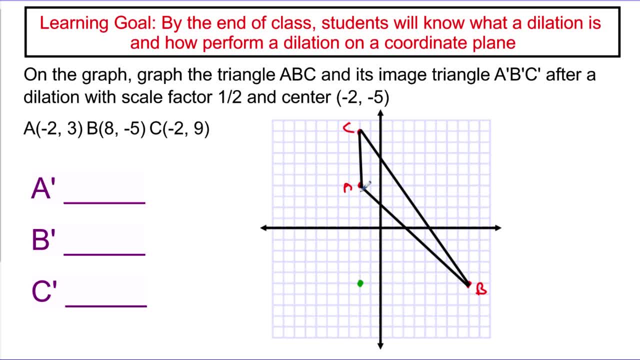 So I have to make sure that the distance between my center and my new A, my A prime, is going to become half the distance, because my scale factor is a half. So instead of being 9 units up, I'm going to cut the distance in half and say 1,, 2,, 3,, 4, and a half. 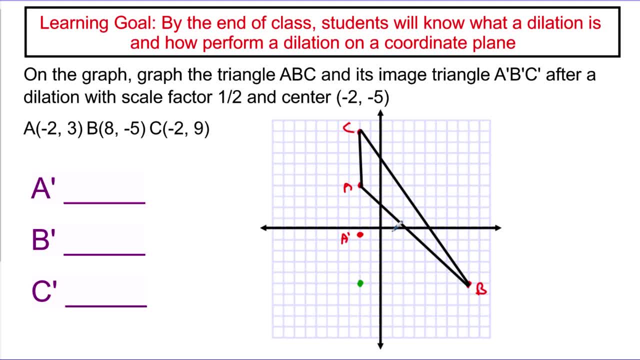 It would be right here and I'd call this my new A prime, So that looks like the point: negative 2 and negative a half, Negative 2, and I'll call it negative 0.5,. OK, And I'm going to do that for each of them.